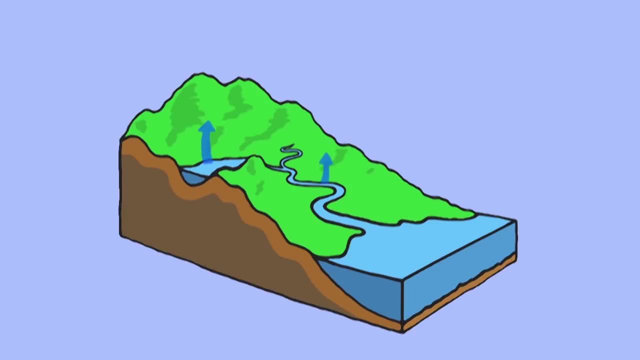 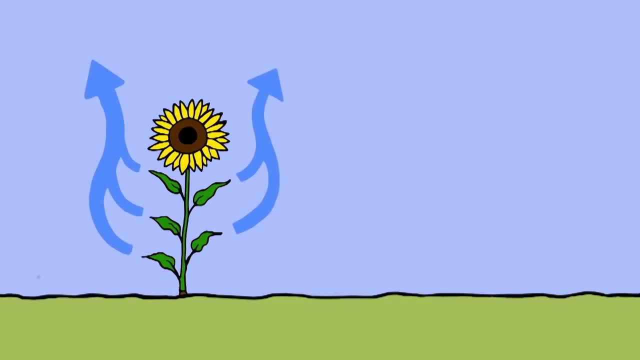 lake, from lakes to rivers and from rivers to seas. All of these act as bodies of water that can be evaporated. The water is turned into a vapour and goes into the air. An unusual source of water comes from plants. Plants transpire. Essentially, this means lose water from their leaves. Similarly, 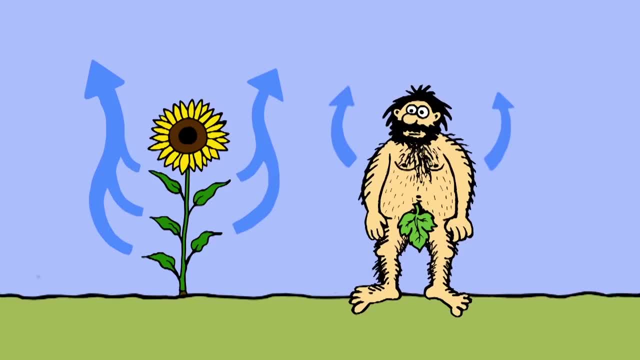 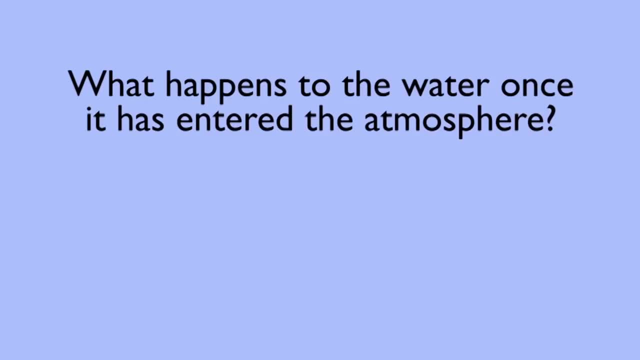 animals, sweat or perspire. All of these processes cause water to evaporate. Once the water has entered the atmosphere, what do you think happens next? Pause the video and continue when you think you have an answer. The correct answer Is that the water vapour cools and condenses. When it does this, it forms clouds. You can. 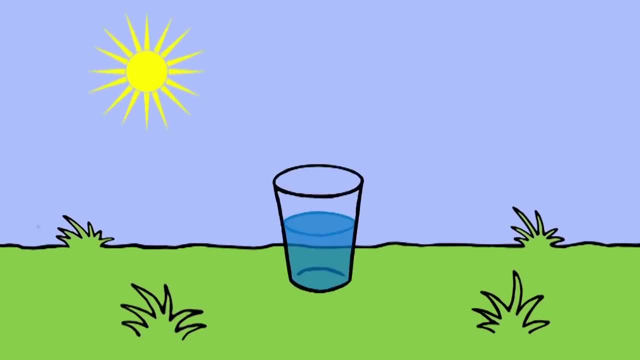 see this effect for yourself. Take a cold glass of water and place it outside. Water vapour will condense on the outside of the glass. The water does not leak through. It came from the warm air and is condensed on the outside of the cold glass Once all of 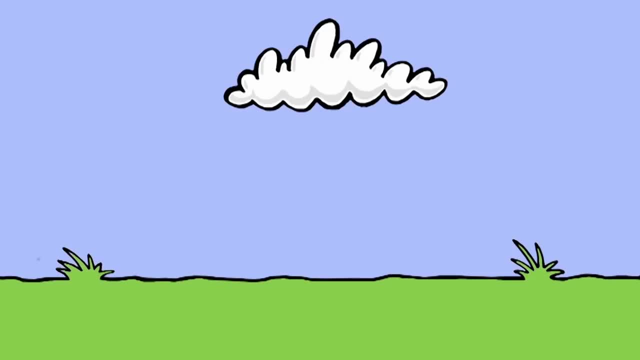 the water is collected in the cloud, you know what happens next? It falls back down. Once all of the water is collected in the cloud, you know what happens next? It falls back down. A fancy word for this is precipitation, and it can take many forms. Can you name a few? 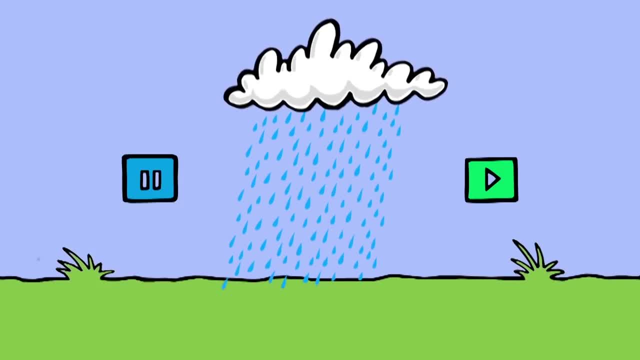 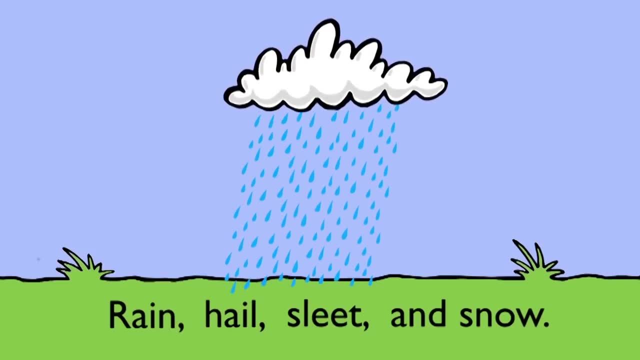 Pause the video and continue. when you can name at least four forms of precipitation. The correct answers include rain, howl, sleet and snow. For those of you who live in warmer climates, howl is condensed irregular ice crystals. Sleet is a term used to describe 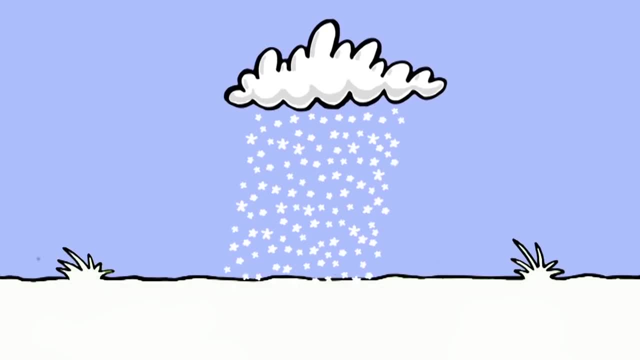 a mixture of snow and rain. Finally, snow is a form of crystallized water. Howl is condensed. irregular ice crystals. Sleet is a term used to describe a mixture of snow and rain. Howl is condensed. irregular ice crystals. Sleet is a term used to describe a mixture. 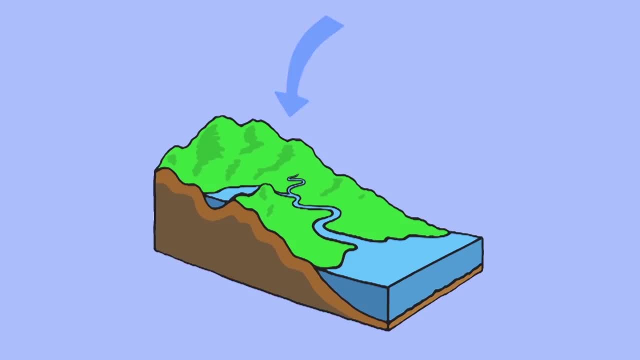 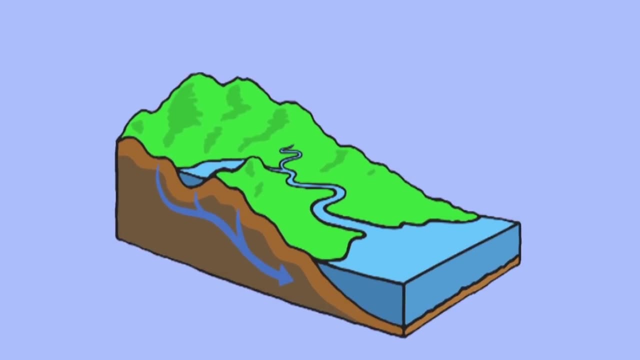 of snow and rain. In the end, the water is collected. It can be collected on land, where it either soaks back into the earth, becoming ground water from which plants and animals can drink, Or it may run over the soil, collecting in lakes, oceans and rivers Where, you guessed it? the 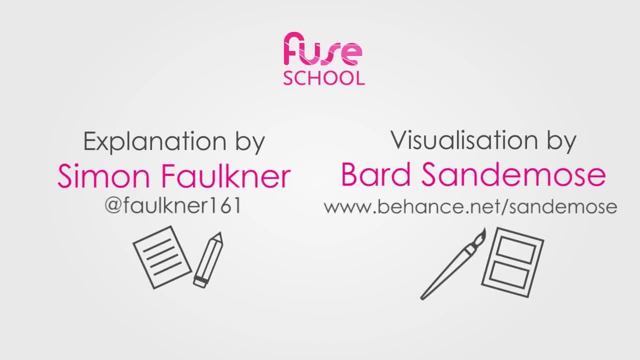 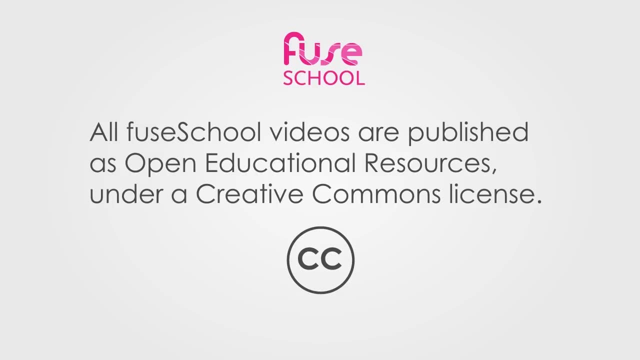 water cycle then repeats Howl is condensed. irregular ice crystals. Sleet is a term used to describe a mixture. you